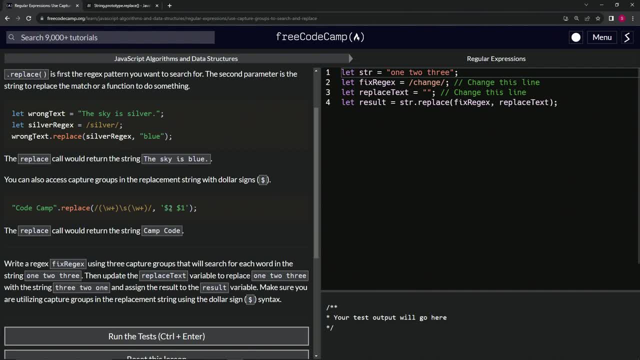 of them. And then we say a string with dollar sign two and space dollar sign one. So this dollar sign one is referring to this one And now it's putting it in the second position. and the dollar sign two is referring to this one And it's putting it into the first position, Right? So the replace 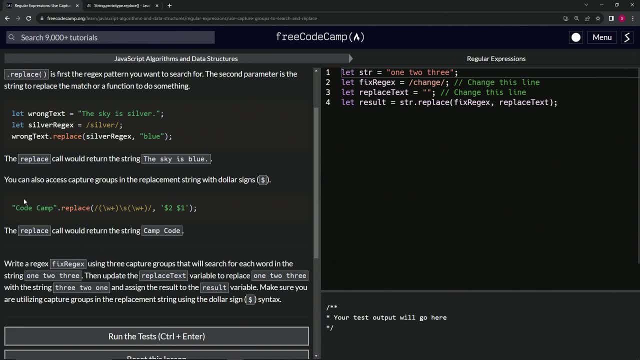 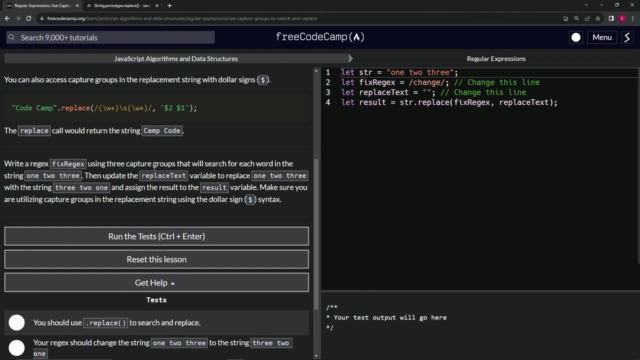 call would return the string camp code. So we put code camp as camp code, like that. So now we're going to write a regex- fix regex- using three capture groups that will search for each word in the string one, two, three. then update the replace text variable to replace one, two, three. 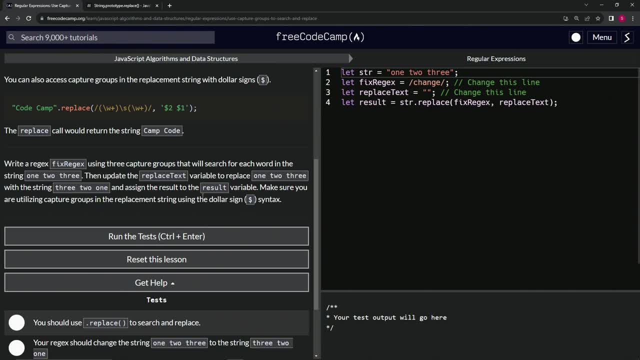 with the string three, two, one and assign the results to the result variable. We're going to make sure we are utilizing capture groups in the replacement string using the dollar sign syntax, All right, So basically, we're going to do exactly like this. We're going to have 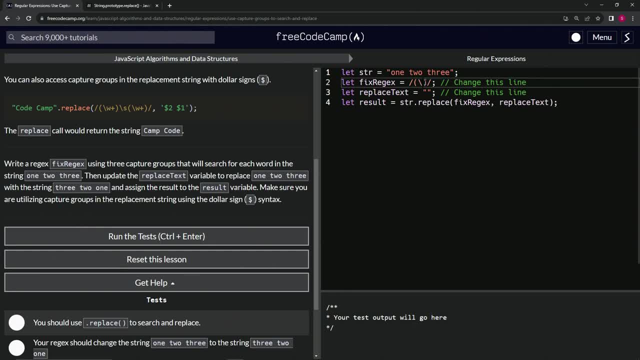 the capture group with the backslash W, And then we don't need to put the backslash S, We can just put a regular space right there, And then we're going to do another capture group with the backslash W. Let's just take this, copy it, paste it and then do another paste like that, And so. 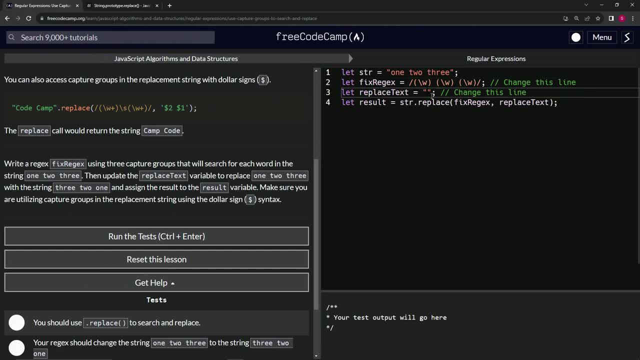 we've got one, two, three like that, And what we're going to do here is we're going to say dollar sign three, So dollar sign three. And then we're going to say dollar sign two- Whoops, not like that. And then inside here we're going to say dollar sign two after a space. 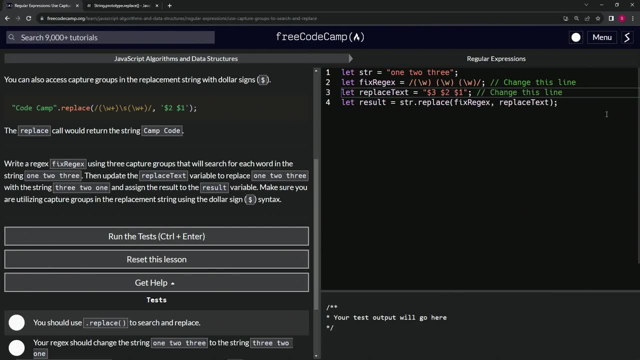 and then another space dollar sign, one like that. Let's come down here and say consolelog results And it says one, two, three. That's not right. Come on now. Do we have to put the backslash S's? Oh, don't forget the plus signs. Right, right, right. So let's add the plus signs after these W's. 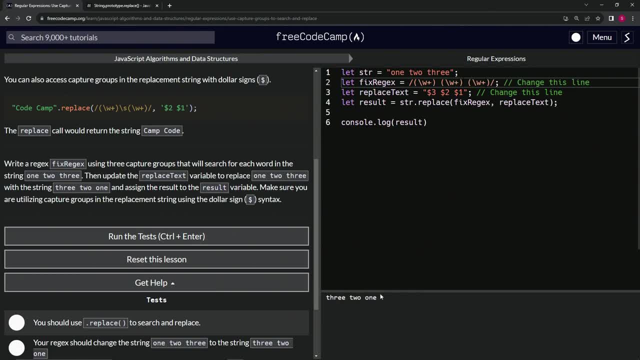 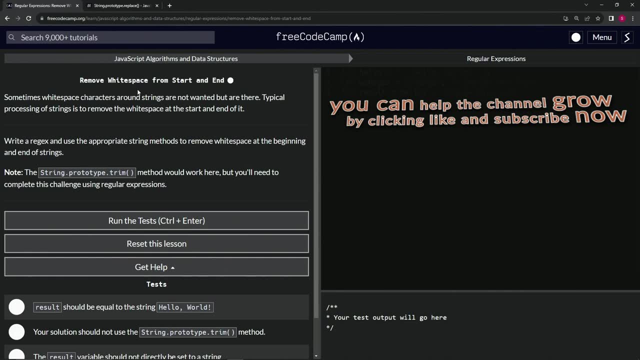 Plus and then another plus And it says three, two, one. Okay, there we go, There we go. So let's run the test- Looks good and submit it All right. Now we're on to remove white space from start and end, And. We'll see you next time.